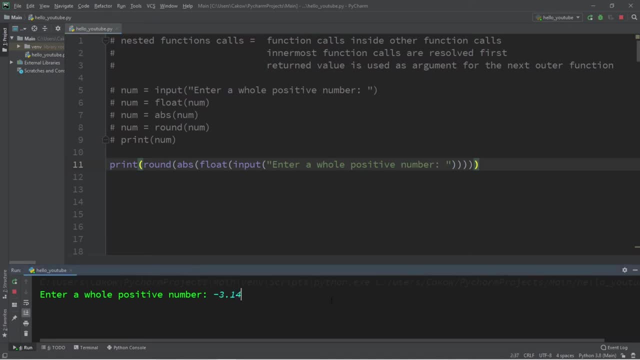 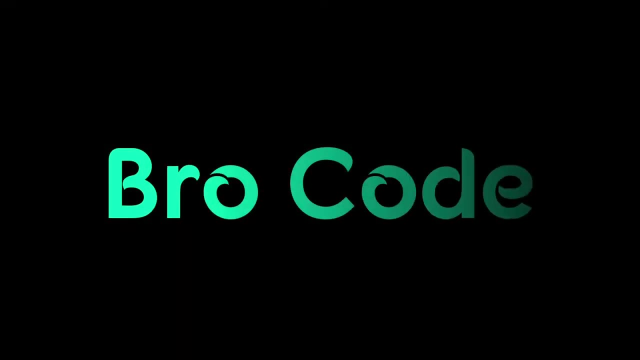 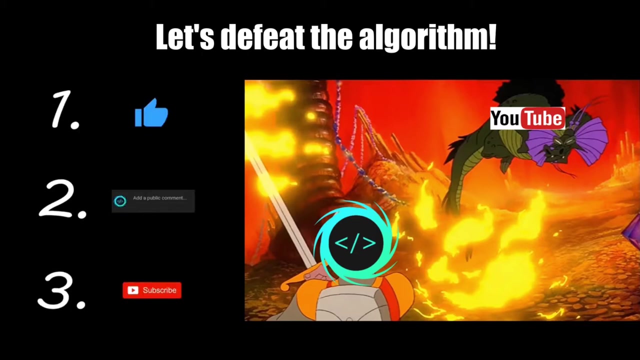 Hey, what's going on? everybody, It's your bro, Hope you're doing well, And in this video I'm going to explain nested function calls in Python. So sit back, relax and enjoy the show. If you find this video helpful, please remember to like, comment and subscribe. Your support will help keep this channel running. 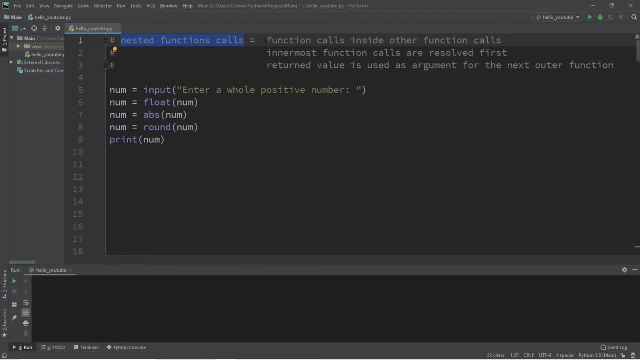 All right, people, Nested function calls. These are function calls inside of other function calls, And this is possible because certain functions will return a value and we can immediately use that value as an argument for the next function. So here's an example. Let's say that we have this small program where we will ask a user to type in a whole positive number, And let's say I don't. Let's say I type in negative 3.14, and then I'm storing that value within a variable named 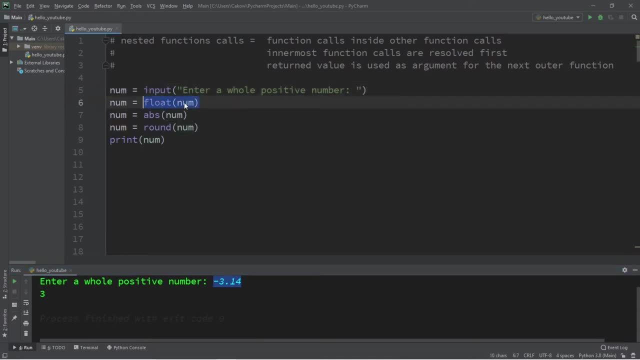 num. What I'm going to do is convert that number to a floating point number, because currently it's a string. When you accept user input, I will find the absolute value of num and then round it to the nearest whole number and then print the value. So we can actually do this using less lines of code with nested function calls. So let's start with the first function which will be accepting some user input, the input function. So this will be in the very center of our nested function calls, And then the next function we will 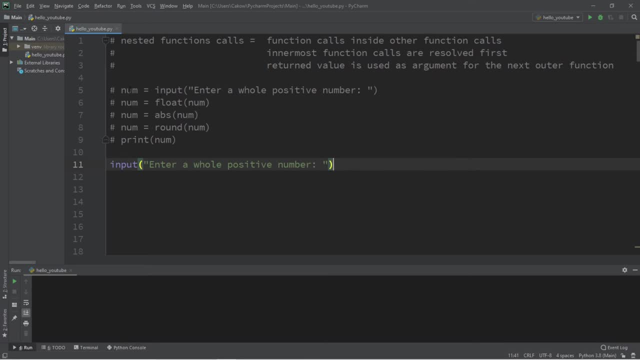 like to apply to the variable that is returned. the value that is returned we will pass in as an argument to our next function of casting this data type to a float. So we'll surround our function with another function and use the float function And then we'll just keep on adding layers to this. So we have the absolute value function next. So we'll add another layer And we have the round function. So we'll add a layer to that And last, 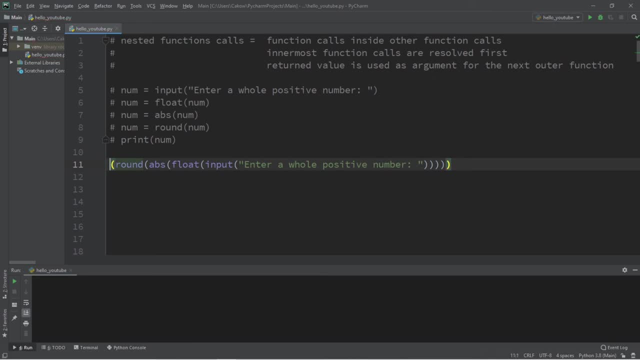 we're going to print And that'll be the outermost layer. So this program will do the exact same thing. Let's say, negative 3.14.. Except we've written this with one line of code. So basically we start with the innermost function and resolve that first. whatever value is returned we use as an argument to the next outermost function- And in this case it would be float- then we resolve that, then move on to absolute value, then round and then print. So it's. 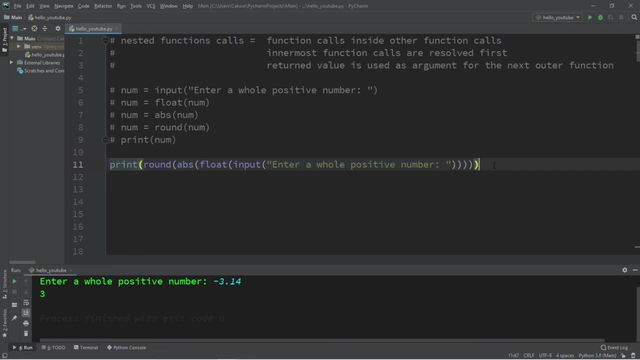 just another way of writing code that takes up less lines, But this is more of an extreme example. you probably won't see like four or five nested functions. Well, everybody, those are nested function calls. If you would like a copy of this code, I will post all of this to the comment section down below. But yeah, those are nested function calls in Python. 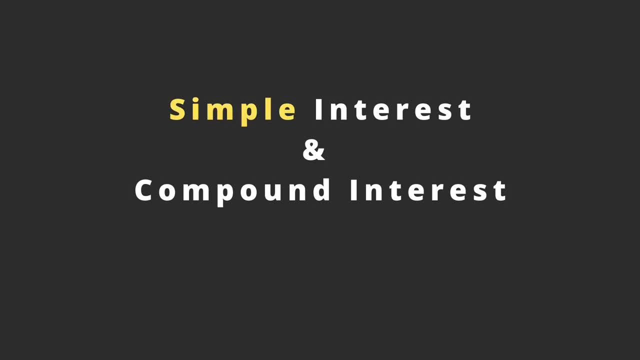 Hey guys, today we're going to go through different problems for simple and compound interest, which actually has a lot of real-world examples and applications. For example, if you put your money into a savings account at the bank, they will pay you what's called an interest for. 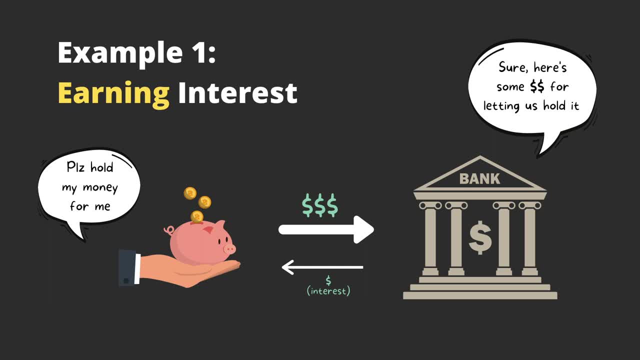 keeping your money with them. They're basically saying thanks for choosing us and letting us handle your money. here's a little bit of extra cash for banking with us. This money that you get from interest, you get to keep, which is basically free money, But on the other hand, if you borrow, 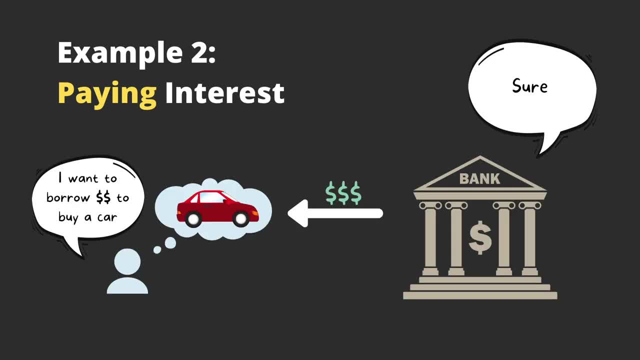 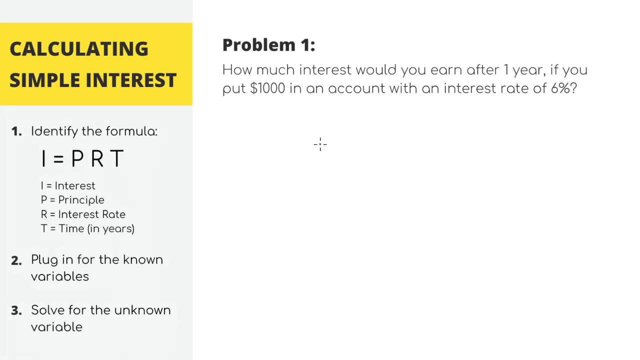 money from the bank. for example, if you took out a loan when buying a car, they will charge you an interest, or in other words, a fee for borrowing their money. This is money that you have to pay on top of what you originally borrowed. All right, let's look at some word problems. 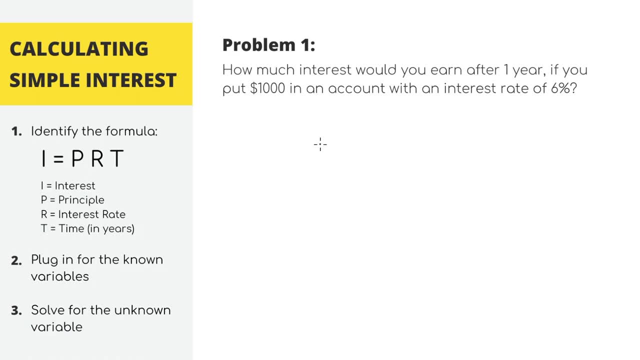 How much interest do you earn after one year if you put $1,000 in the bank with an interest rate of 6%? There is actually a formula you can use to calculate interest. It's: I equals P-R-T, where I is the amount of interest or money that you'll earn. 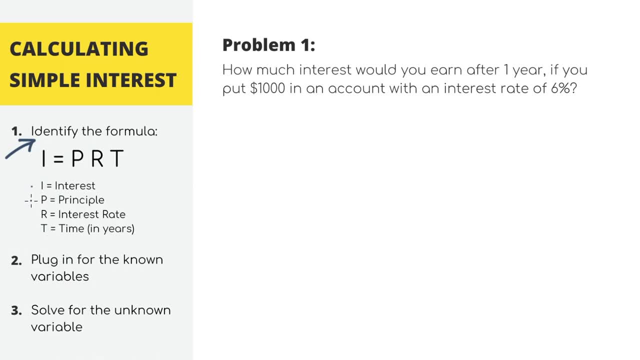 P is the principal, which is the amount of money that you first put in, R is the interest rate and T is the amount of time that you first put in. 15% is the first people's interest. 50% is the interest rate and it means the amount of time. 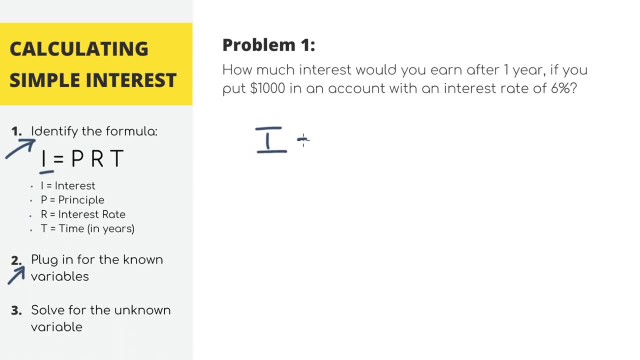 your money is in that account in years. So for a problem we are trying to find, I, which is the interest we'll earn, P is the principal, or in other words the amount of money we first put in, which is $1,000..